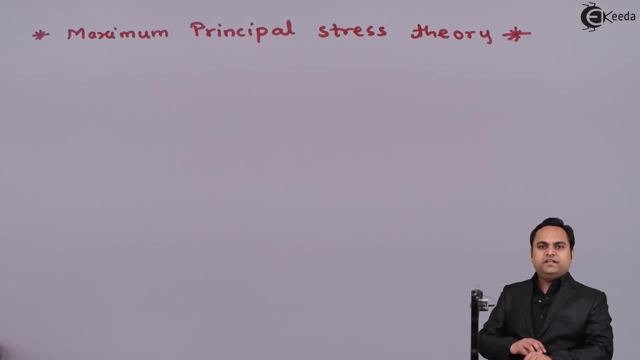 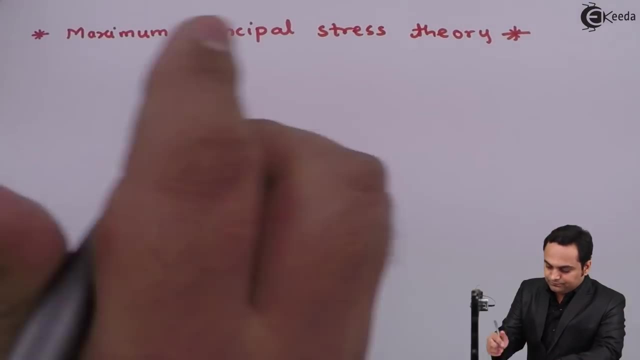 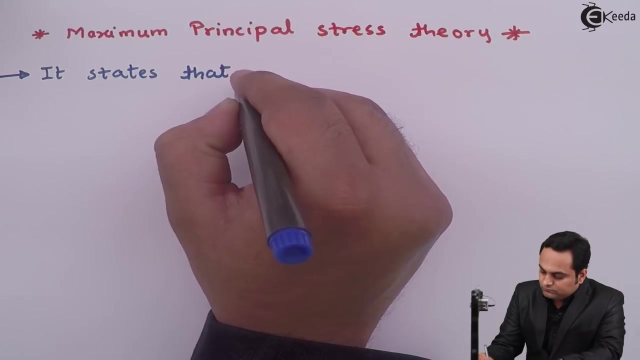 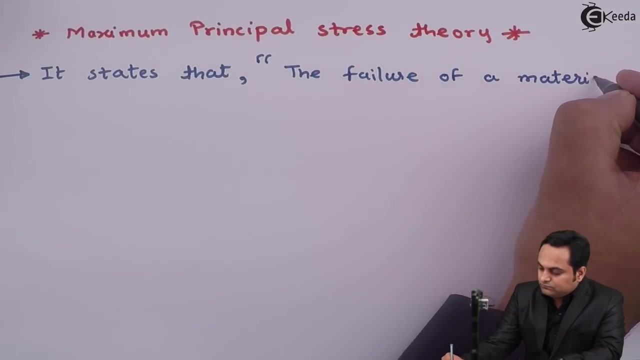 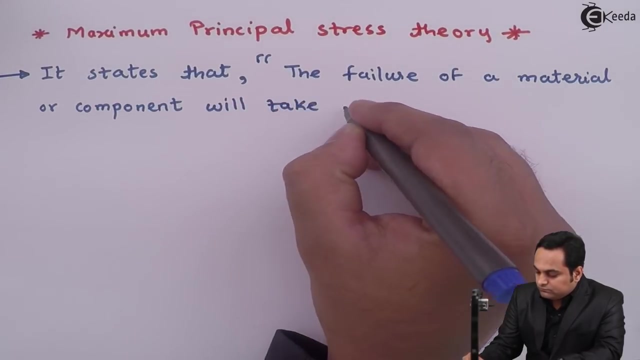 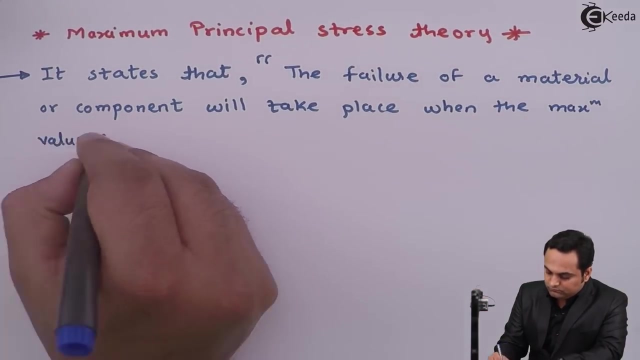 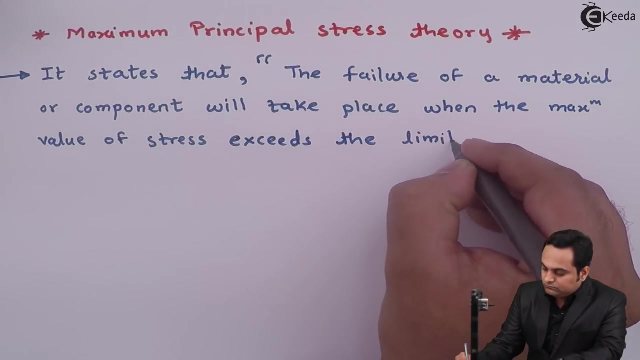 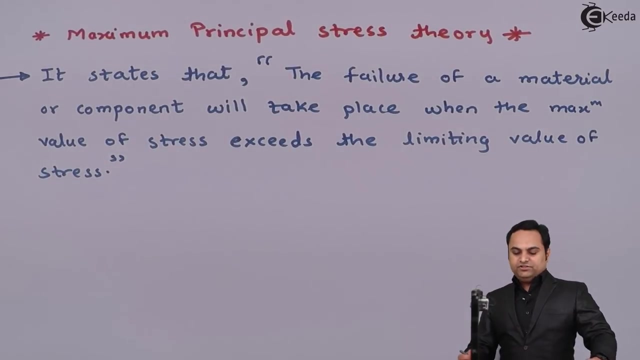 So it means this theory basically deals with tensile or compressive stress, And it states that here I will write the statement of that. Now, here I have written the statement for maximum principal stress theory. It states that the failure of a material or a component will take place when the maximum value of stress exceeds the limiting value of stress. 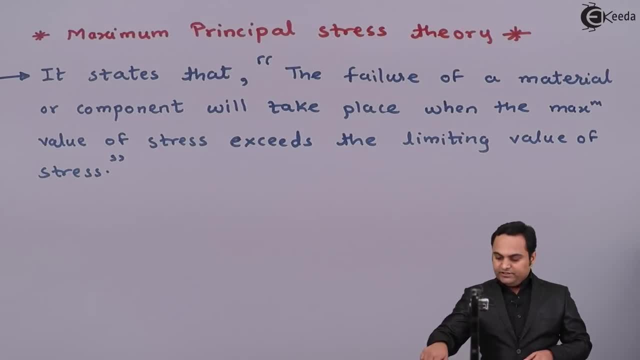 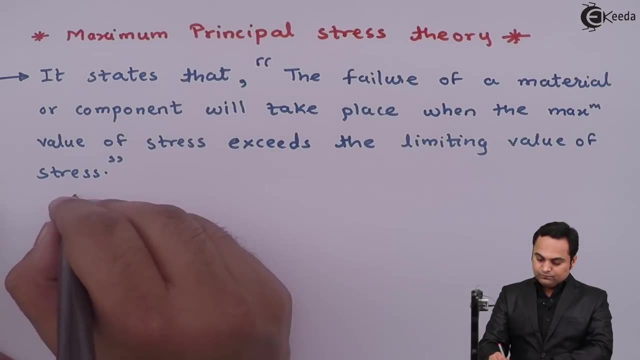 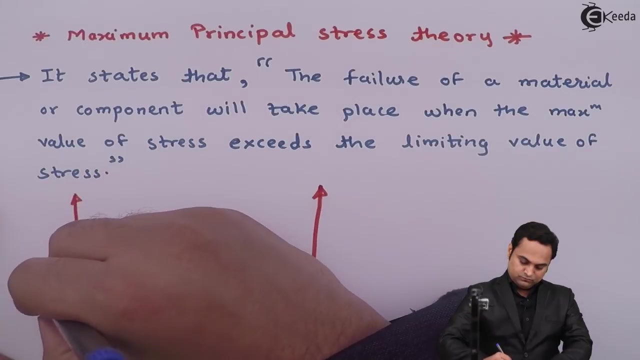 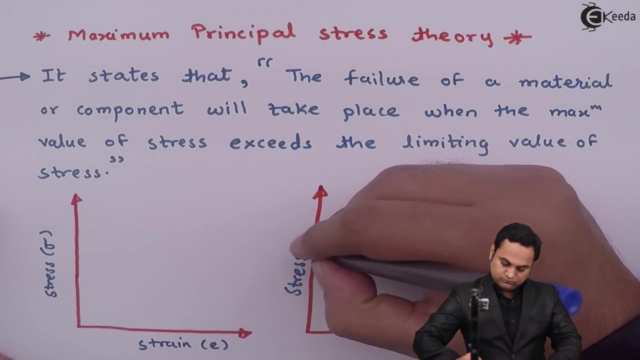 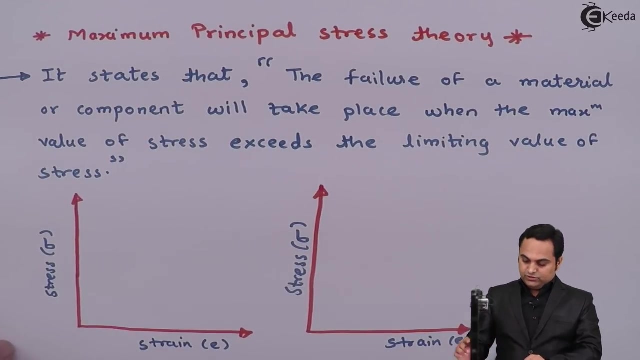 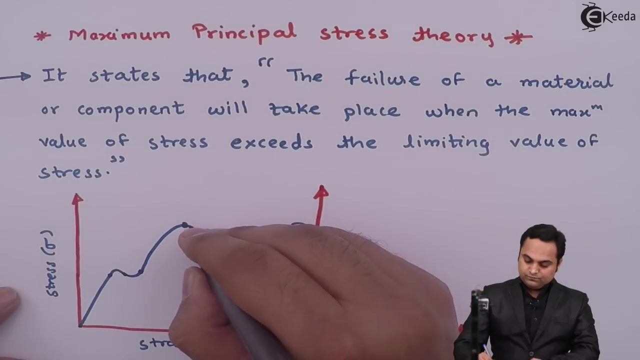 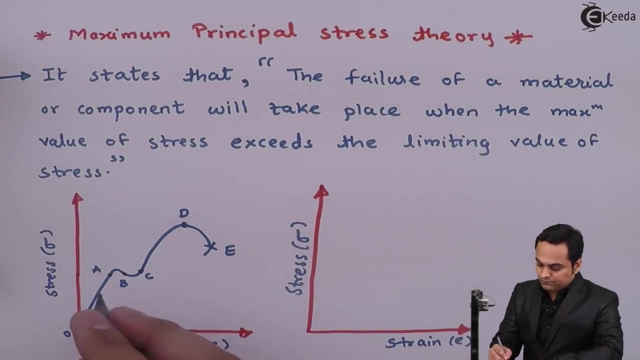 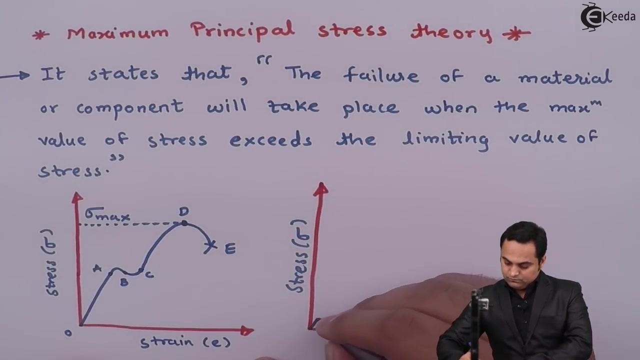 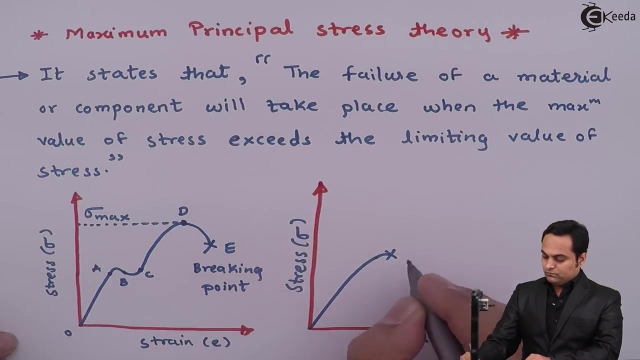 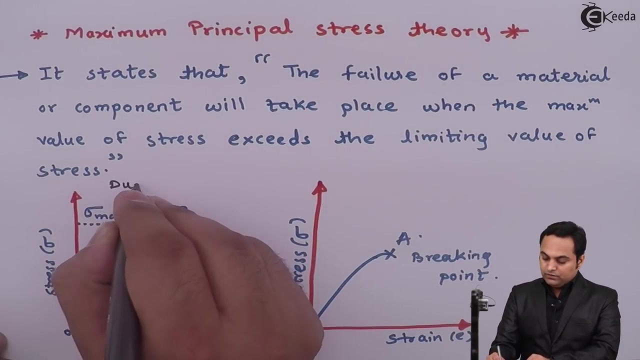 Now let us try to understand what is the meaning of this by drawing a diagram. Now here I will draw two stress-strain graphs. First, the first one. Now here I have two different graphs. The first graph which I have drawn, it is for ductile materials- 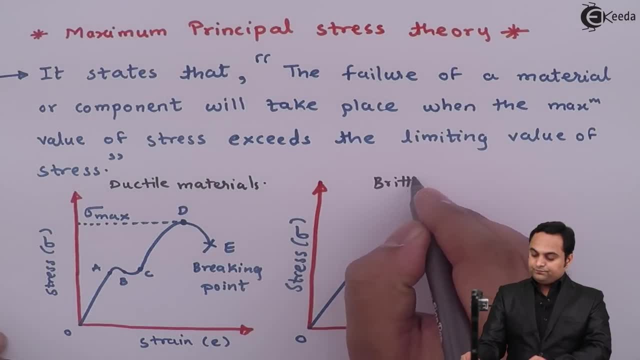 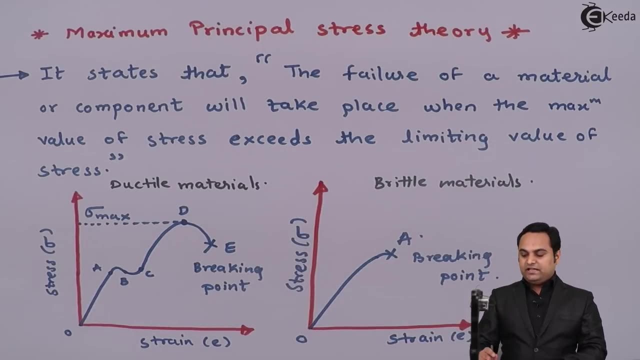 And the second one which I have drawn, it is for the ductile materials. And the third one which I have drawn, it is for brittle materials. Now, as we can see in the first graph, that is for ductile materials. 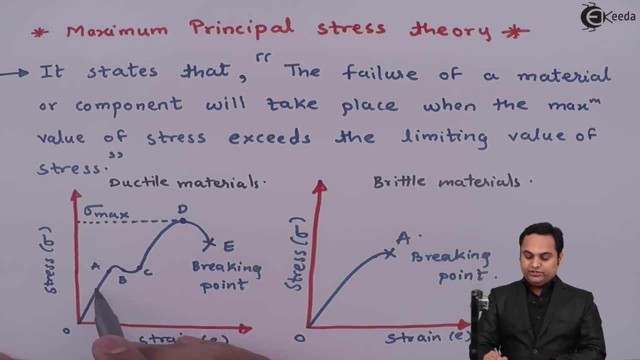 when we are increasing the stress, strain also increases, And there is a point in this graph, that is point D, where we are having maximum value of stress. Now, from this graph it is clear that after the maximum stress has been reached, 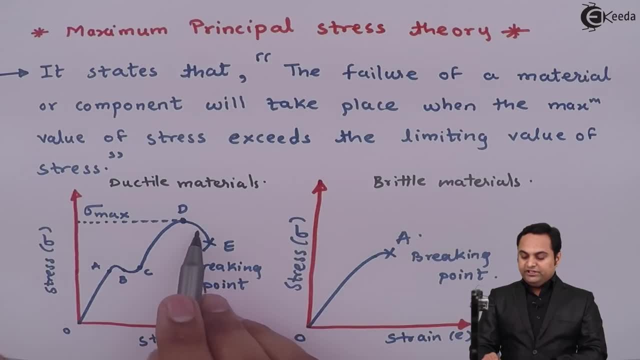 then there is increase. So there is a region from D to E in which, even if the stress goes on decreasing, the strain value increases And finally, at point E the material breaks. So if in any material the value reaches the maximum value of stress, then after that maximum value has been reached, 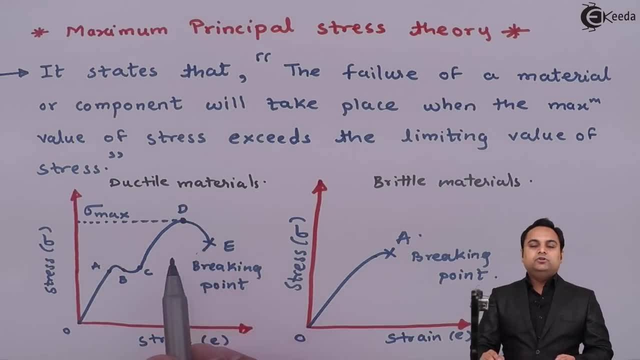 that material can break anywhere. So the chances should be to avoid the material to operate in the maximum stress condition. We have to reduce the working stress so that the material does not reach maximum stress. So this is for ductile material. 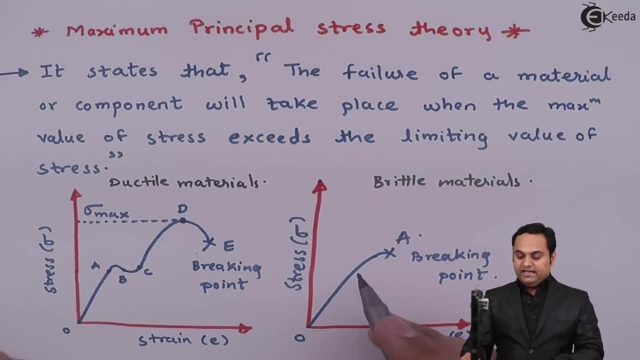 Next, check it for brittle material. Brittle material, as we know it fails without giving any prior warning. So when we are increasing the stress value, the strain increases And finally there is a point where the material breaks. 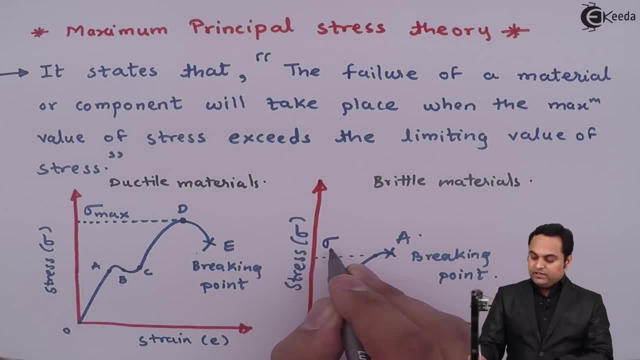 And at that point the stress is called as sigma, ultimate stress. That is ultimate stress. So, as per the definition or the statement of maximum principle stress theory, here we have written that it states that the failure of a material or a component will take place. 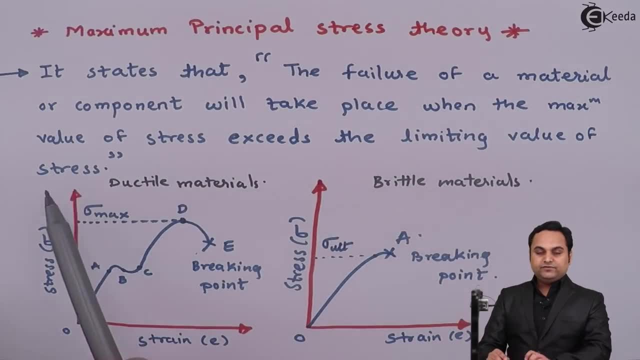 when the maximum value of stress exceeds the limiting value of stress. The limiting value of stress is here the maximum stress, And then if we are increasing the stress from this value, that is, point D has been reached. then the material can fail anywhere. 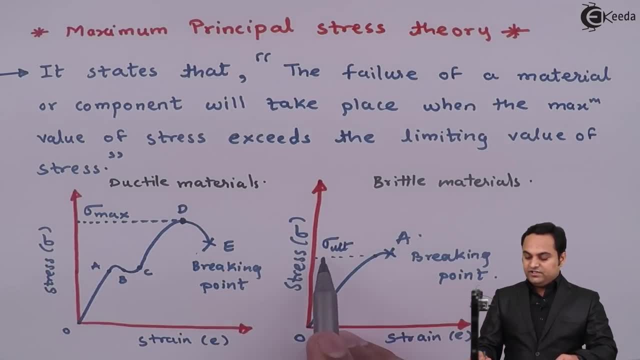 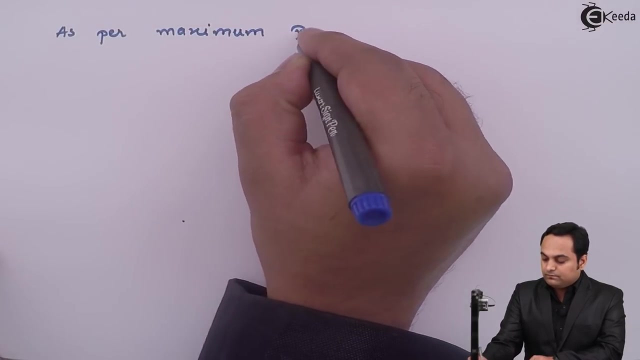 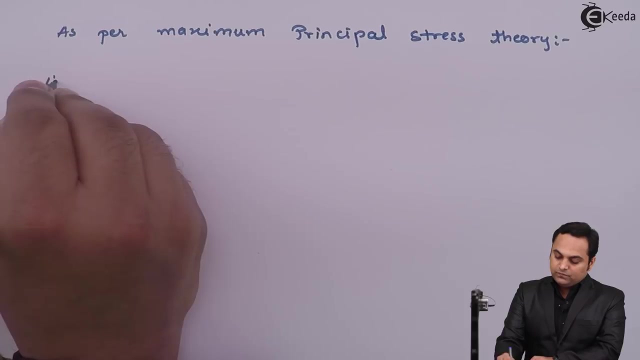 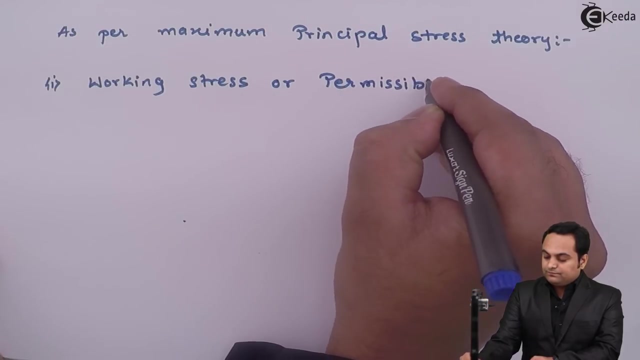 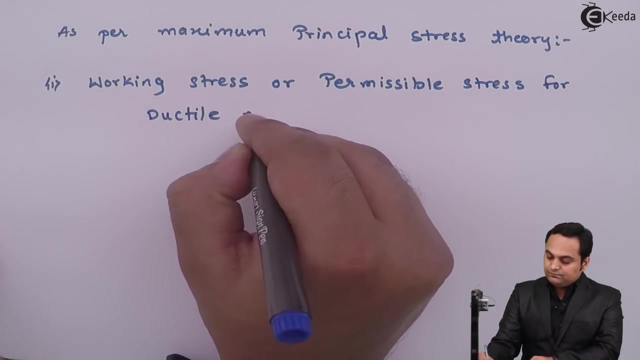 Similarly for brittle materials. as we can see, if the material has reached ultimate stress value, then it can break anywhere. So, as per the maximum principle stress theory, as per the maximum principle stress theory, working stress or permissible stress for ductile materials. 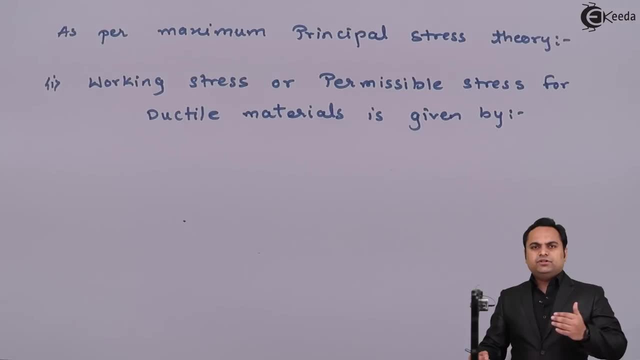 is given by. we need to reduce the value of working stress so that it doesn't go into the maximum stress condition, And for that we have to use factor of safety. that is the permissible stress. I'll write down sigma: permissible.